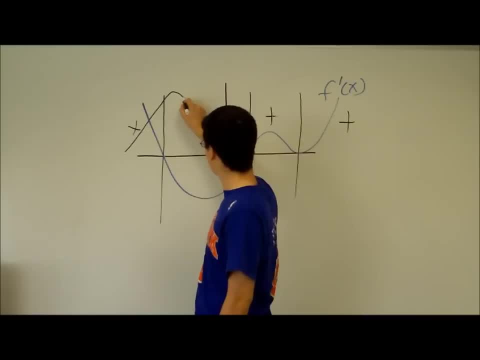 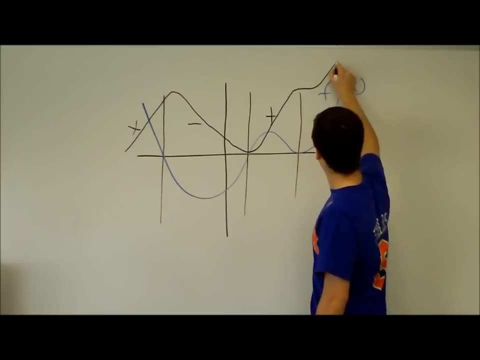 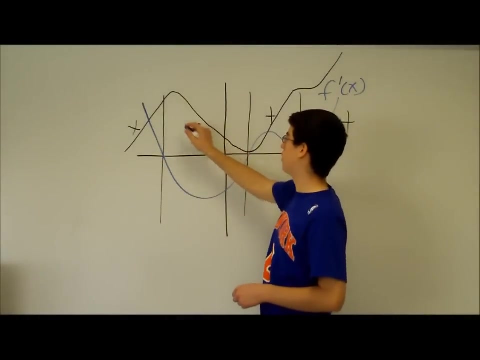 right, That is beautiful. So you have a positive slope. I think you want to go just up to that line and then the slope should be flat. right about, I think you went a little far with that, but that's fine Yeah. 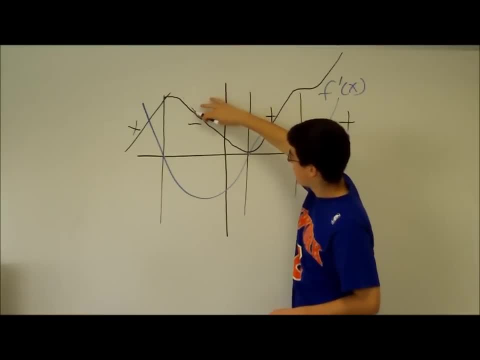 That's fine. So the slope goes down for the whole negative and then up and then up again. So that's a sketch of the original function. So why don't you label where the critical points would be? You're off by a teeny bit, right. It should be right on that vertical line that you drew. 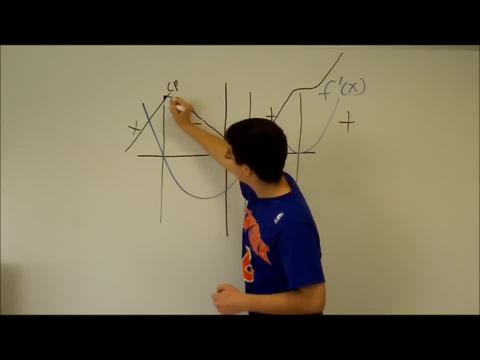 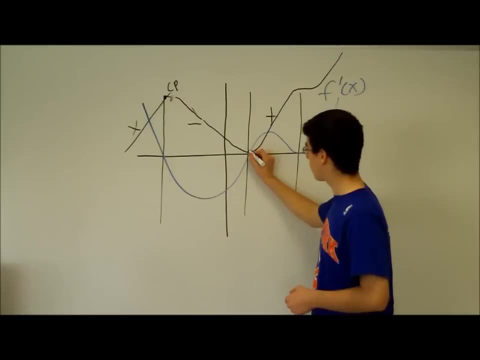 Oh, yeah, Yeah, because that's where the Fabulous- And I think you're off a little teeny bit on the- Is that the? Oh no, you're right, You're right on there. Look at that, Oh, how's. 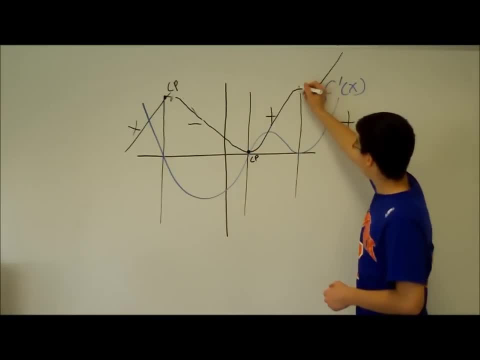 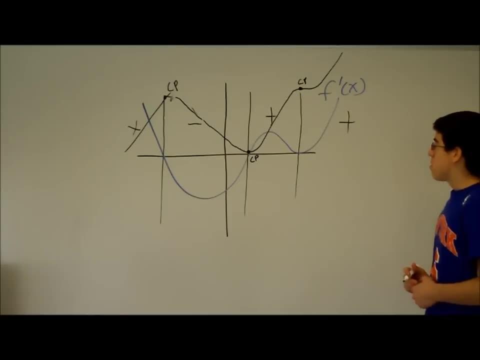 this messing up? Jeez, All right, It's in zero, The slope is zero, Fabulous. So those are placed where the slope is zero and you can figure out where the maximums and minimums would be on the original function. So I think you have a max and a. 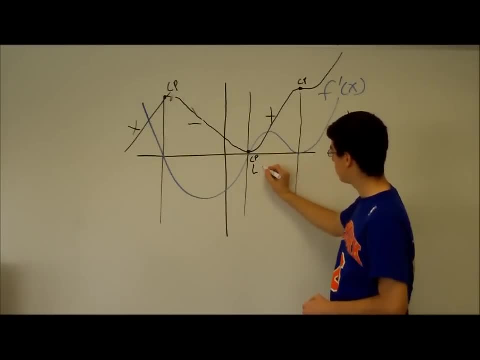 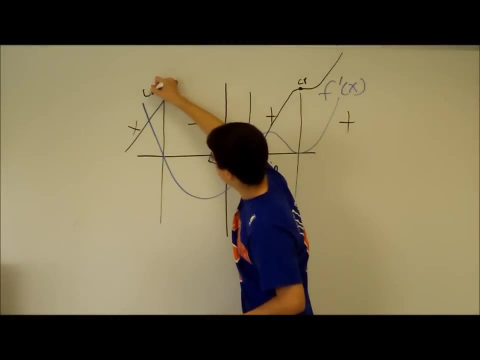 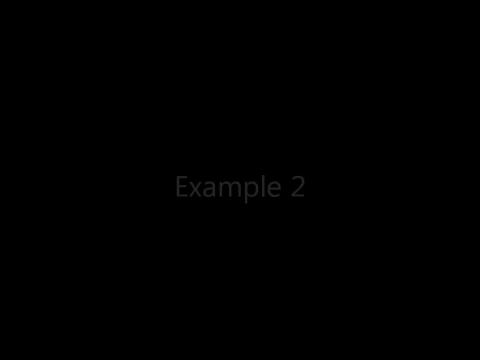 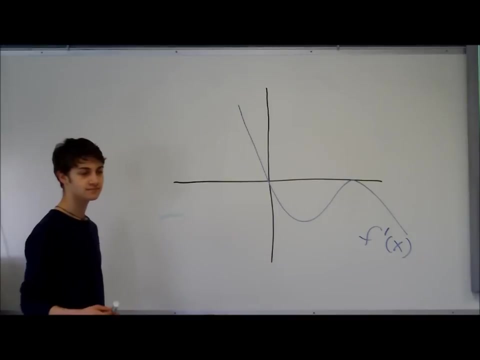 It's working good. Thank you very much. All right, So we have Sam here and that's a picture of the derivative, and you're going to sketch the original function and find the critical points Any time you want, You're okay. 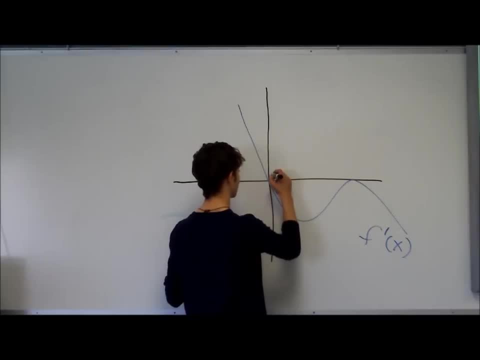 Thanks, Sam. So what do those vertical lines represent? It's where y prime is zero. Ah, so that's where the y value of the derivative is zero. that's fabulous. So then you, like, wrote the function into three, right? 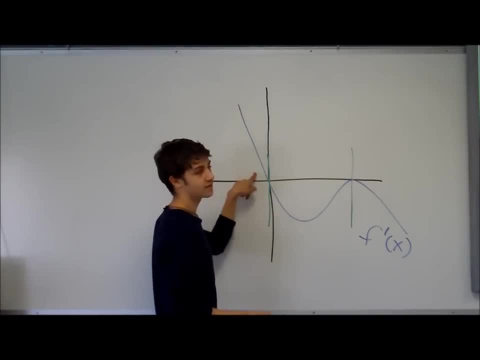 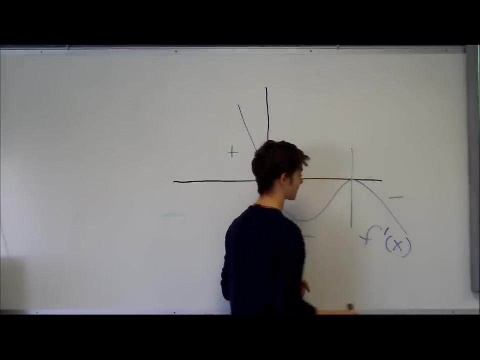 Okay, So the y values in this part are positive. Nice little plus sign there, okay, And here they're negative, And then negative here. So the y values of the derivative represent really what Slope, Slope of the original function. 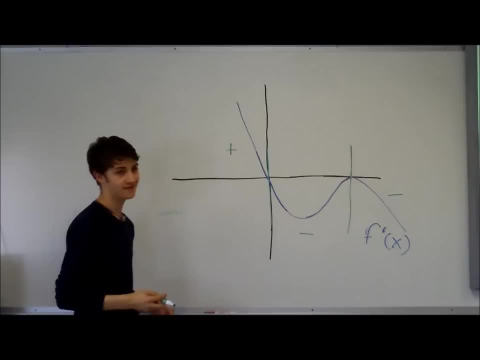 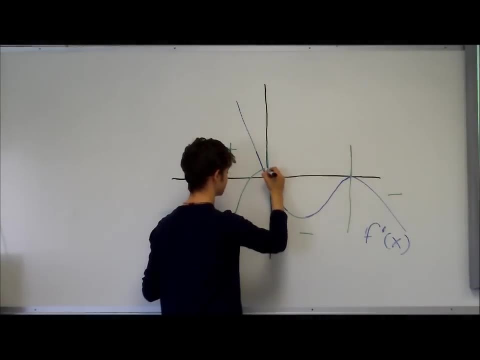 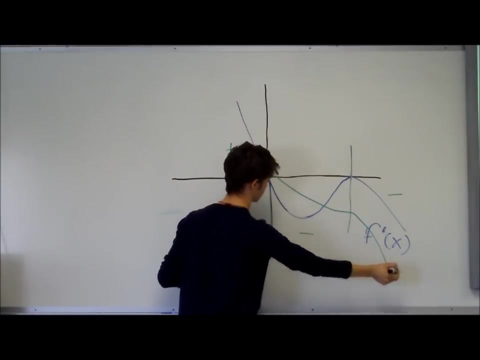 That's fabulous. So sketch the original function. All right, Sam. so yeah, okay, go ahead. So uphill until the green line- fabulous. And that minus means negative slope, And then negative slope forever and ever. Yup, so you have two critical points. 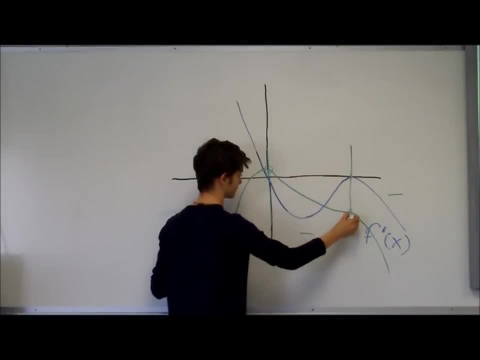 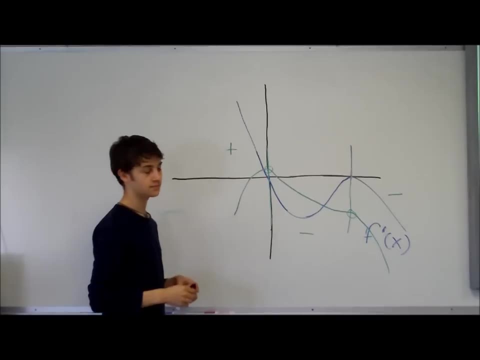 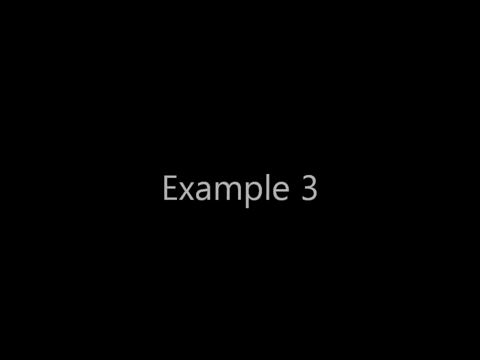 And you have a maximum. Which one's the max, That one, And is there a? what's the other critical point? Neither max or min. Fabulous, all right. Thank you very much, Sam. Thank you, You have Seth here. 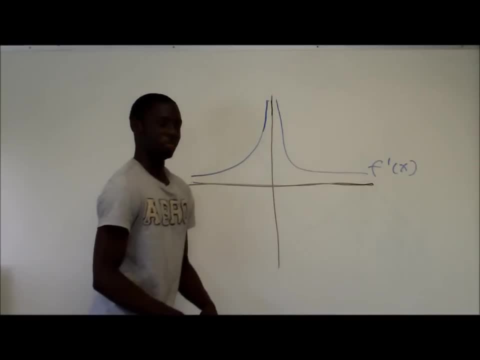 You're going to sketch a function based on its derivative, And this one's a doozy here, so You can do it. Sketch the do's there, Seth, Come on. So you're looking at a derivative. Now hang on. 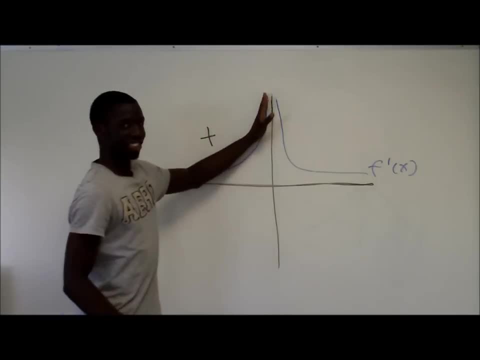 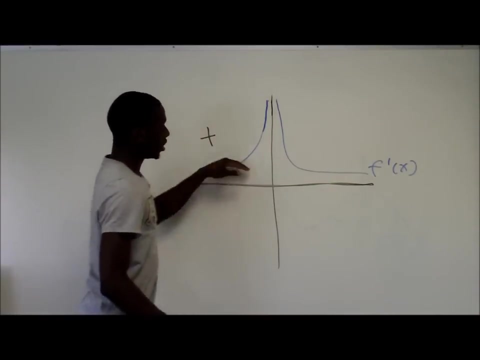 So what do those pluses mean there? Well, but why did you? you put a plus because? Why did you put a plus there? Because the y values- thank you, Sam, the y values- are positive. And how about on the other side of the yeah. 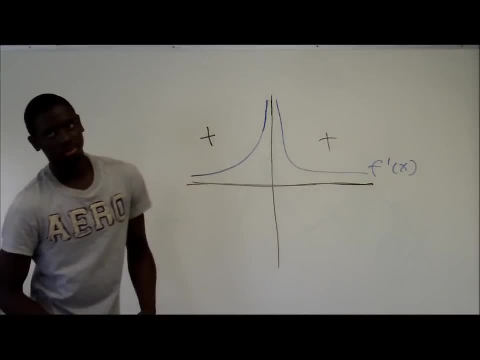 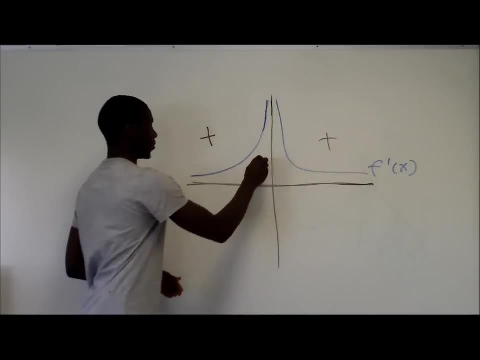 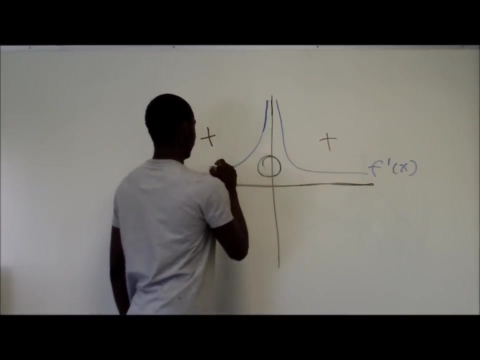 So this derivative always has positive y values. And is there a place where this derivative is undefined? Right in the middle? Beautiful. So sketch the original function. Okay, It's got to have a positive slope, an undefined slope- I see you're sketching- and a positive slope again. 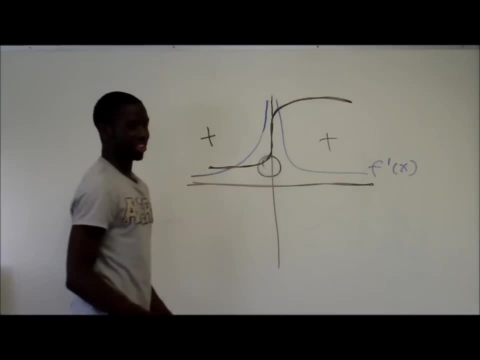 How's that look Beautiful, That looks fabulous. All right, Thank you, Seth.